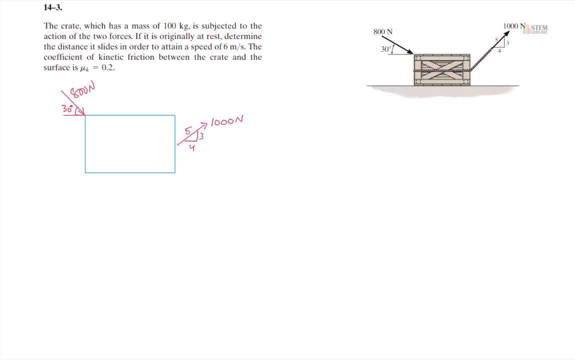 that's at that 3,, 4, 5 triangle. All right, now notice it says that we've got friction in here, So we need to include that. So if we're pulling it to the right right, notice you know this force. 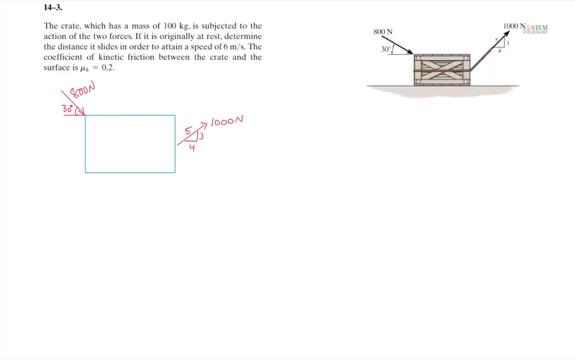 obviously is going to be moving this way. So friction is going to go in the opposite opposite direction. So it's going to go like that And we need to put that on here. So here's friction. Remember, for friction you're going to have your coefficient of friction times your 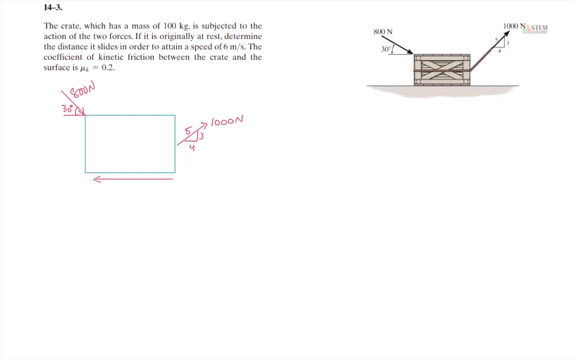 normal force. So for this case we're going to have 0.2 times n. We'll find n in just a minute. Now, n, like we were talking about, is the normal force, So that's just going to go straight up. 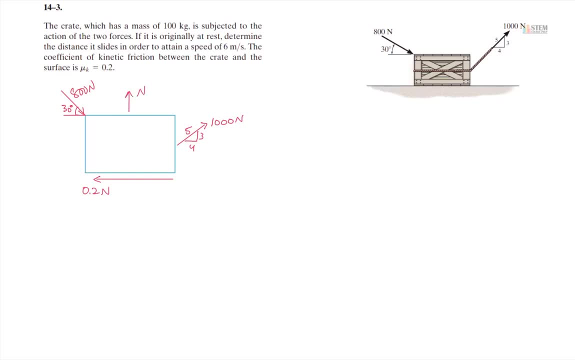 right here. And then last thing we would have would be the weight. All right, so it's going to be 100 times 9.81.. And that's what we've got, All right. so first, in order to get friction, I need the normal force. 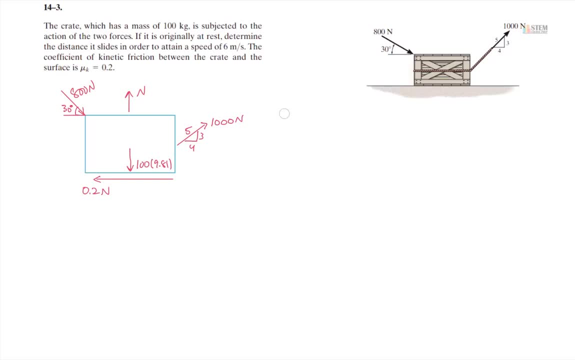 Let's go ahead and calculate that And then we'll look at what's doing work. So to find this, let's just look in the y direction: Up's positive. So we're going to have an n and then minus the weight. 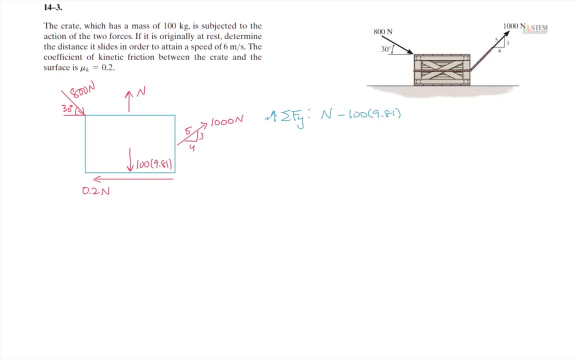 And then this has a y component, as does this. So let's just start here on the 800.. It's going to be a negative 800.. And then we're going to have a y component, as does this. So let's just start. 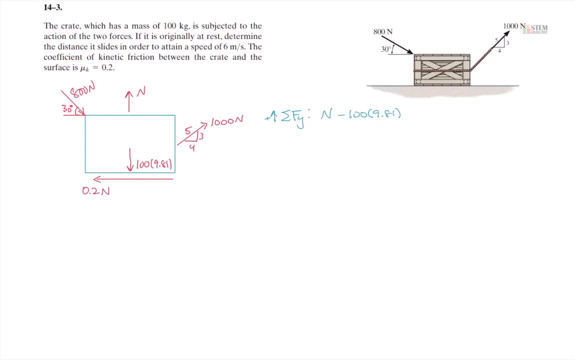 here on the 800, sine 30, because that would be that component right there. So negative 800, sine 30. And then this one over here: well, that's going to be a positive y component, So we're going to put plus 1,000. And then we've got that 3,, 4, 5 triangle. 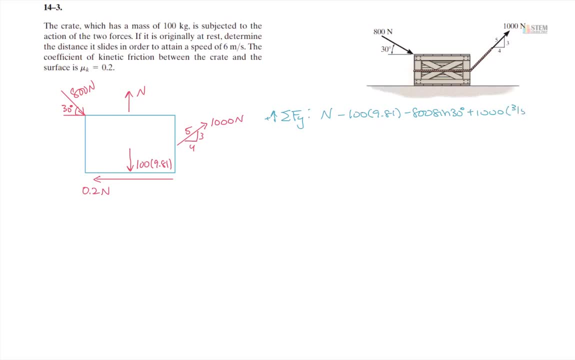 So to get the component, we're going to multiply that by 3 fifths. All right, so we've got that And we're going to set it to 0 because there is no motion in that y direction. Now, if we go through and solve, we're going to get 781 units. here would be newtons. 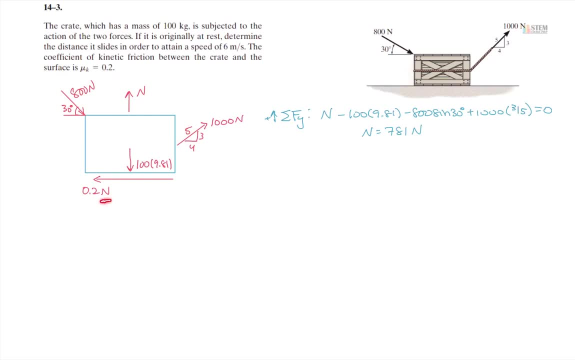 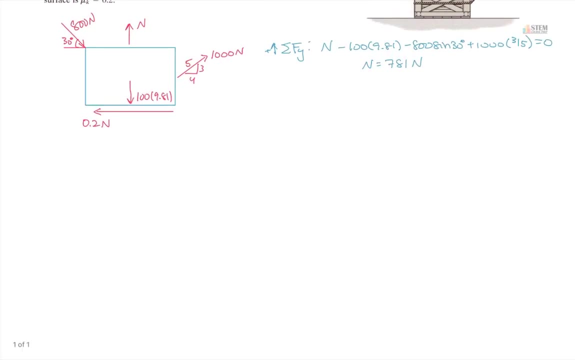 So that's our normal force And we'll be able to use that right here when we do our friction. So now let's look at what forces do work And remember: in order for a force to do work, you have to have the force and displacement in. 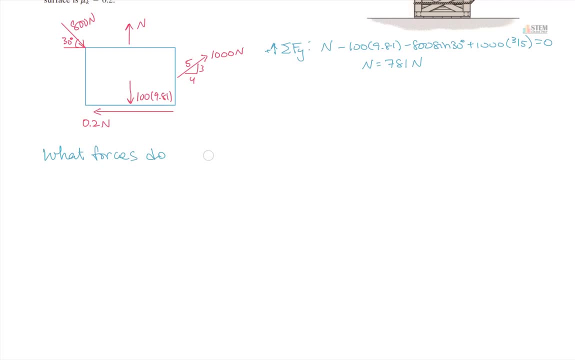 the same direction. Whoops started writing what I was saying. So let's look and see. We know our displacement is to the right, right Horizontal direction. So does gravity here, does weight produce work? No Same thing with the normal force. These two 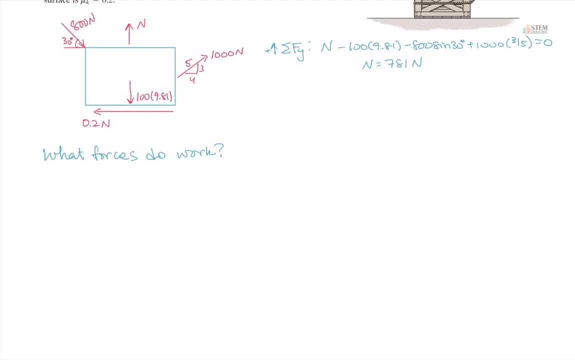 are not doing any work because we are not having displacement in the y direction. right, Our displacement is totally in the x direction. That means friction is going to do work because friction is in the x direction, right, It's in the opposite direction of displacement, but it's still in you. 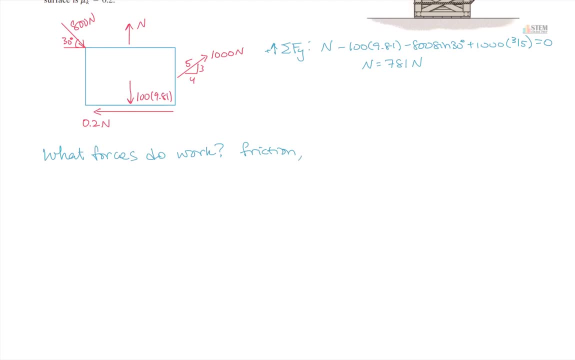 know the horizontal direction right, And then we're going to have this component here That's going to do work. So let's just put the 1000 Newton force, And then same thing with 800, because again there's that x component. So let's put 800 here. Now we've got that figured out, Remember. 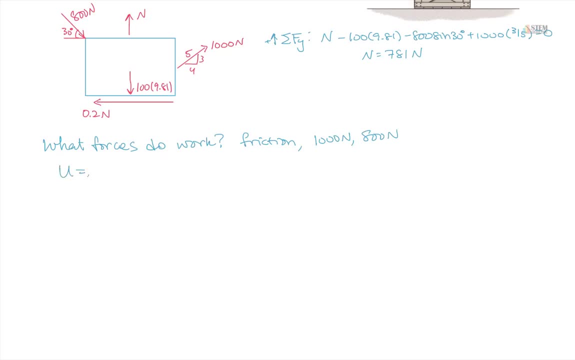 for work energy. we're going to be using the equation: u equals delta t- At least that's the notation for the Hibbler textbook. So let's go ahead and find u. That'll be the total work. So remember it's force times, the displacement in the direction of the force. Okay, so let's go. 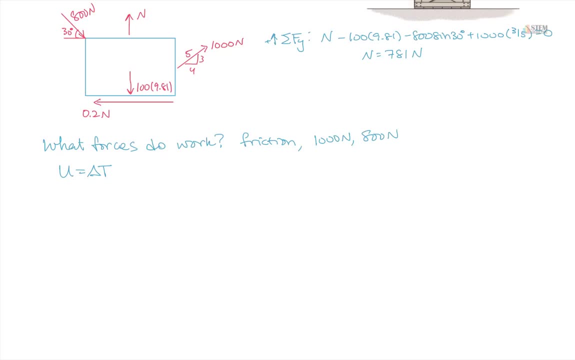 ahead and find that, And then we'll set it equal to delta t, which is the change in kinetic energy. All right, so u is going to be the forces that do you know work, right? So we're going to look at- let's look at- 800 first. So we've got the x. 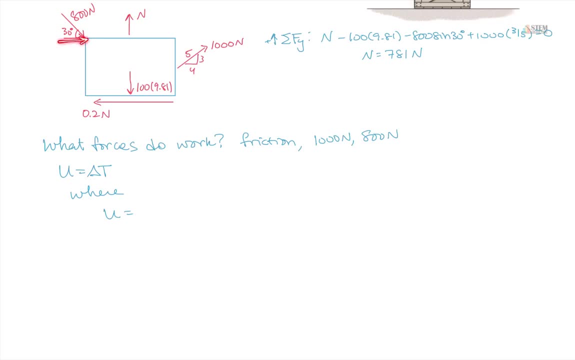 component of this force. It's 800 cosine 30. That's in the x direction. So that'll be our force. So let's write 800 cosine 30. And then I need the displacement in the direction of that force component, right? So the x displacement, I don't know what it is right. That's one of the things. 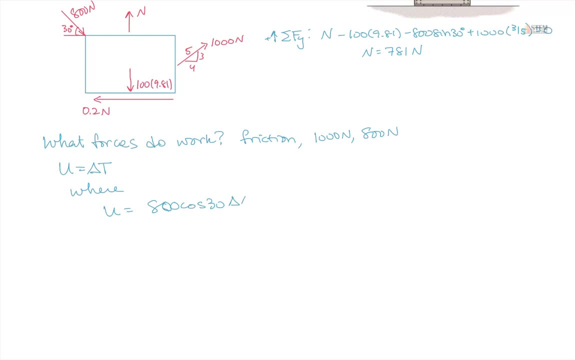 that's what we're looking for, basically. So let's just call it delta x, right, Because delta x is what we're looking for. Now we need to look at the sine. Is it positive, Is it negative? Now, if, 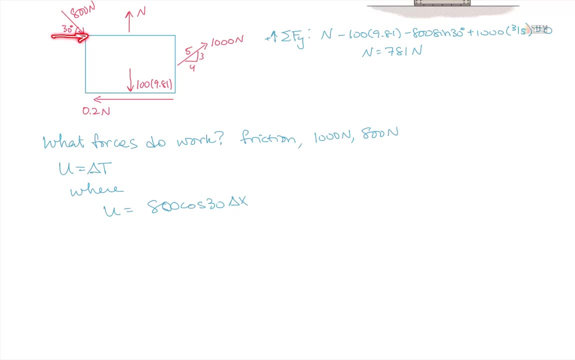 we look, the force component is going to the right and our displacement is also to the right. So if they're in the same direction, this is going to be a positive right. So that'll be a positive work right there. Now let's look at friction. Notice, friction is to the left and the friction 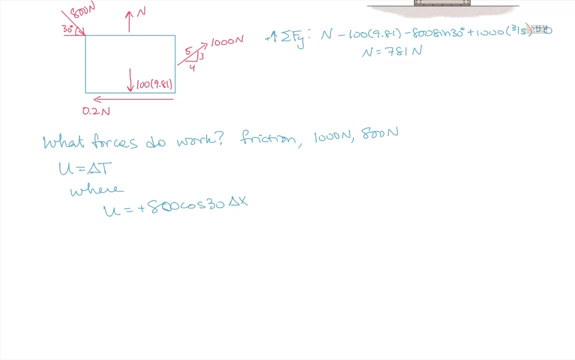 force is 0.2 times the normal force. The normal force is 781.. So let's put that in here. So point two times 781 and the displacement again, we don't know, it's going to be Delta X. now should this one be positive or negative? because our displacement is. 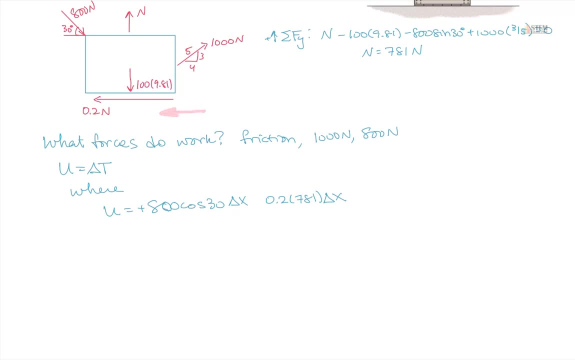 this way, but the force is this way since they're in opposite directions. this is going to be negative, right, and then last one is going to be this X component right here. so that's gonna be the 1,000 times 4 fifths, and the displacement is: 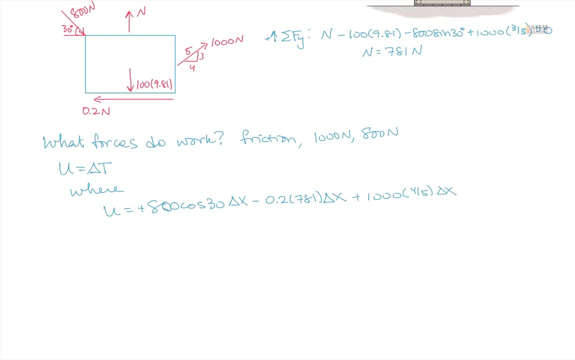 still at Delta X, and this one will be positive, right, because the displacement is this way and then our force component is in the same direction. so that'll be a positive, and then you can go through and simplify all of this. so if you do that, you're going to end up with 1338. 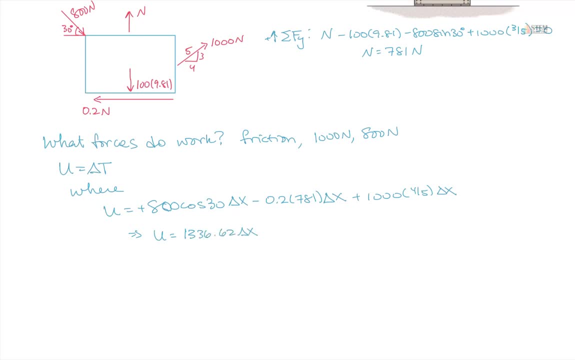 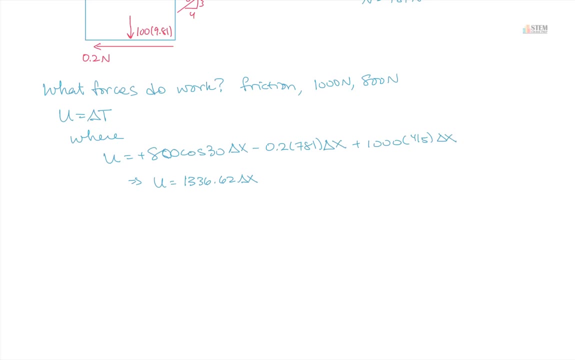 3248.. six point six, two Delta X. and then now we can take that and set it equal to Delta T. remember Delta T is the change in kinetic energy, right? so U is Delta T and remember what Delta T is. it's 1 half times the mass times, your final velocity. 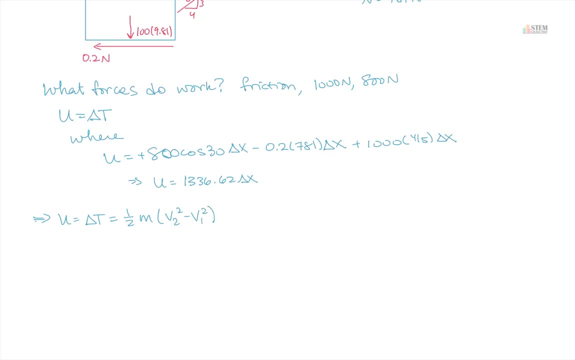 squared minus your initial velocity squared. so now we just basically need to put U on the left here. thirteen thirty six point six two. Delta X set it equal to 1 half times the mass. the mass was 100. and then we need our velocities. so let's go back up and look at the velocities, because I don't remember what. 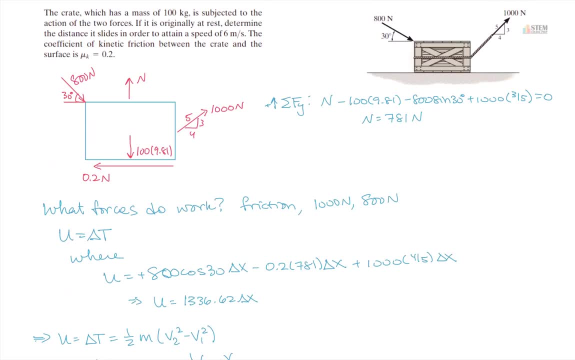 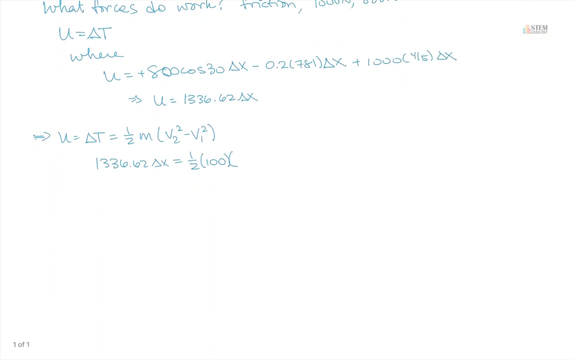 they were okay. so first it's originally at rest. so that means v1. our initial speed is going to be zero, and then it wants to attain a speed of six meters per second. so this is going to be our final speed. so v2 will be six. so